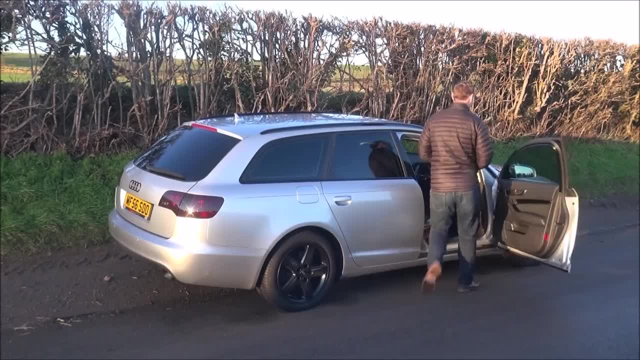 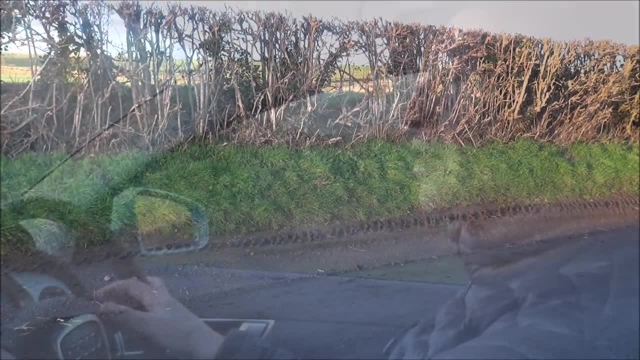 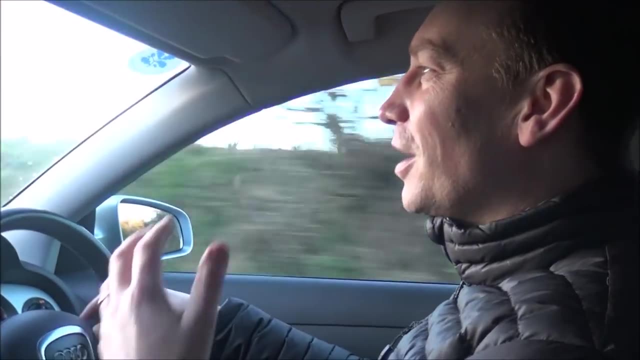 So let's see if it works Now. the key thing about this experiment is that the sound that's being emitted by the moving object does not change its pitch at all, so it doesn't matter how quickly I'm going: the sound of the horn stays exactly the same relative to me. 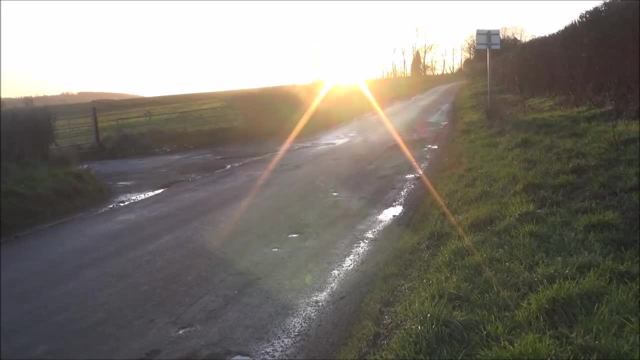 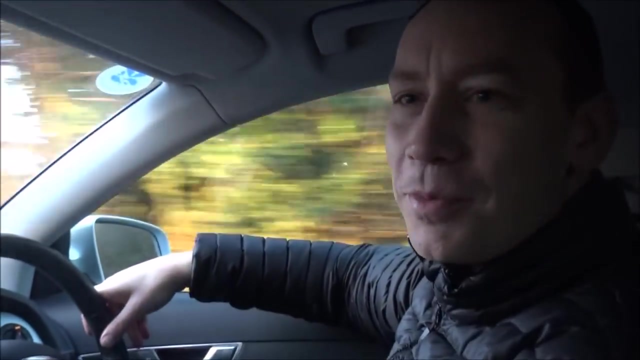 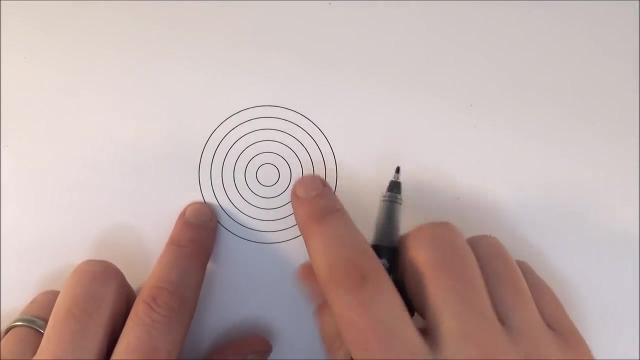 So now it's time for a little bit more theory about the Doppler effect Over to me in the studio. So this diagram here just represents, maybe, the wavefront coming from an object. So there's an object in the middle here and maybe this is sound waves coming out like the car horn, or it might be light. 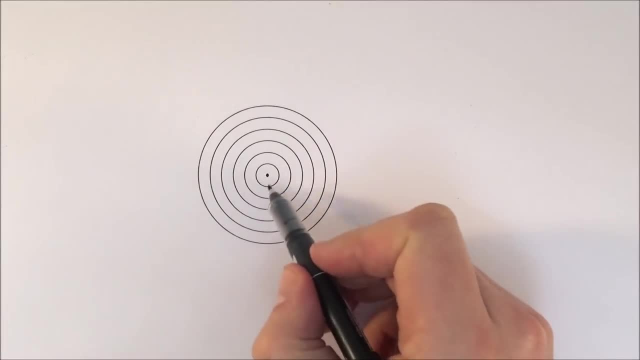 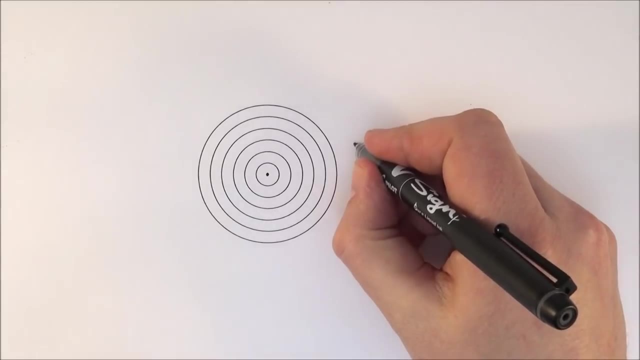 You know, coming off a star or something like that. Now, each of these lines here represents a wavefront, and what these are doing are these are all moving away from the object in the middle, But at this time, the velocity of the object, which I'm going to call v, is equal to zero. 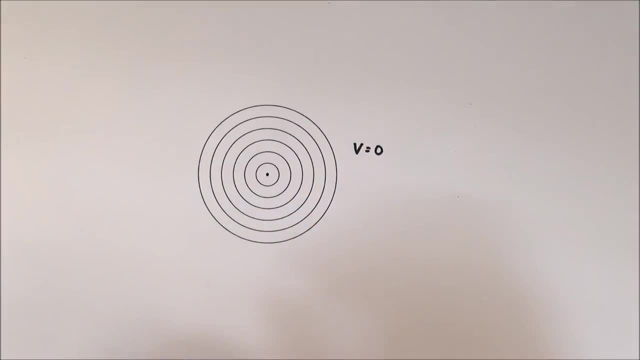 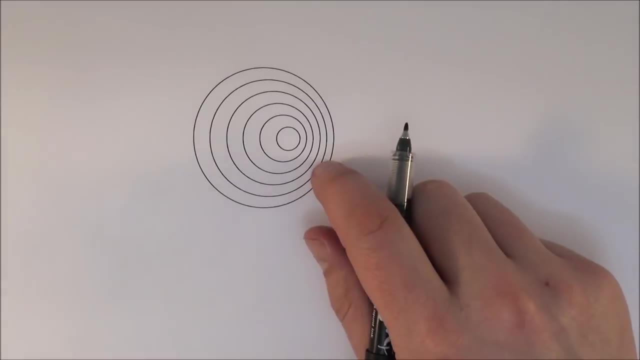 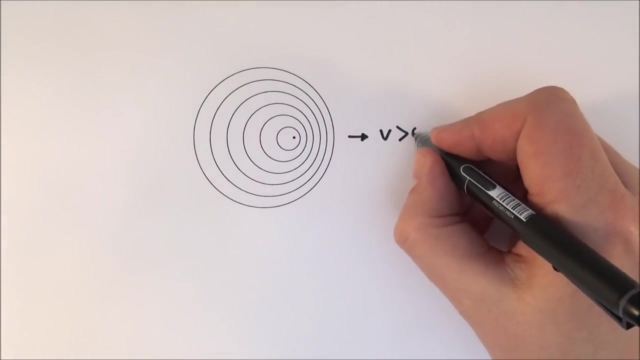 Okay, so this is kind of what happens if something isn't moving. But let's consider what happens when v is bigger than zero. But now here's an object which is maybe moving to the right with a certain velocity of v. This is where v is going to be greater than zero. 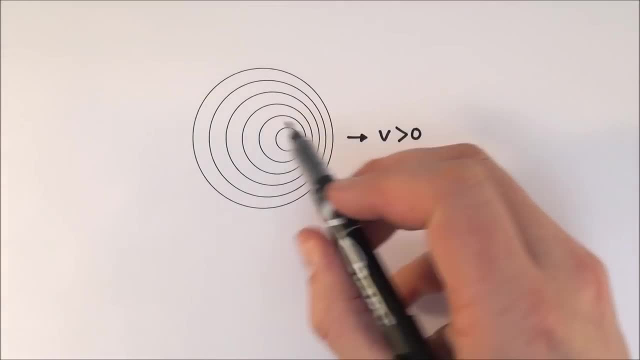 And what we see is that the wavefronts at this side here are bunched up and the wavefronts over here are kind of spread apart. What does that mean? Well, if we look at the wave here, we see that in the same amount of space we have more waves. 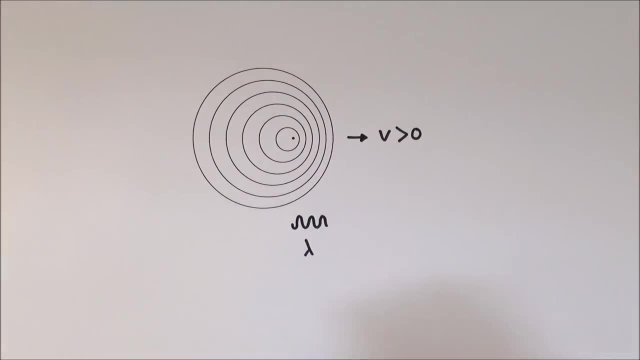 So that means the value of the wavelength lambda has decreased Over here the value because the waves are being stretched out. they've increased so the value of lambda has got bigger Over here. if you had an observer over here, they'd see more wavefronts per second. 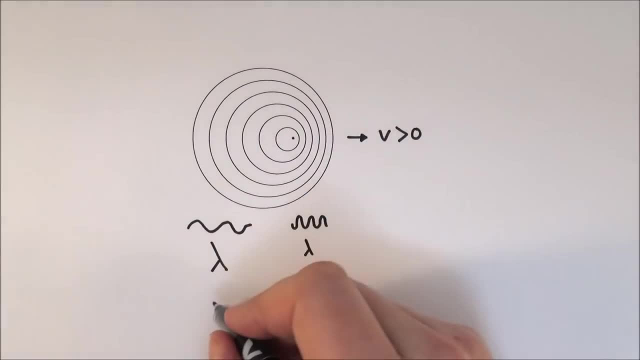 So the value of the wavelength lambda has decreased, So the frequency that they'd observe would increase and over here the frequency would decrease And we saw that with the car. So if we compare the sound of the car when it was stationary, 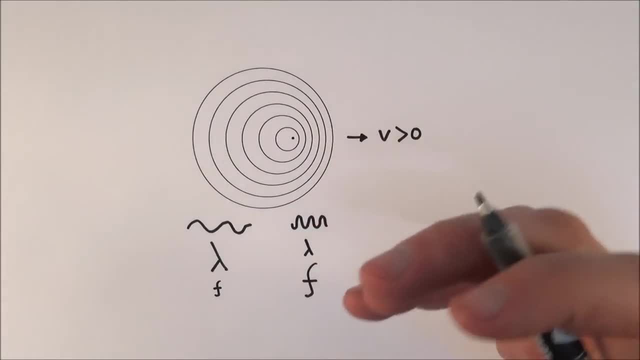 with the sound of the car moving towards us. I think it's quite noticeable actually that you do get a higher pitch and therefore a higher frequency as that object is moving towards you. But let's think about some mathematics, Well, and actually how we can actually calculate, maybe, the change in the frequency and the wavelength. 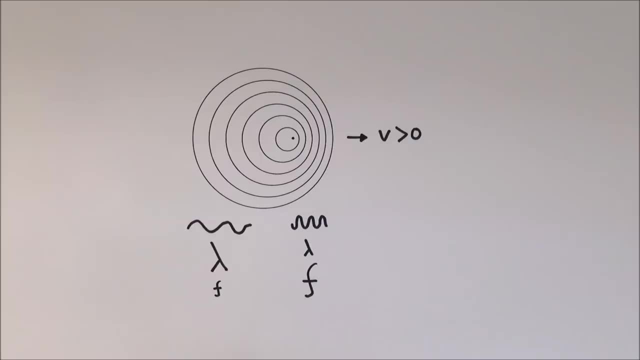 Well, it depends upon not just the value of v, but also the value of c. Now, the important thing here is that c is the speed of the wave in the medium, and v is the velocity or the speed of the object that's moving. 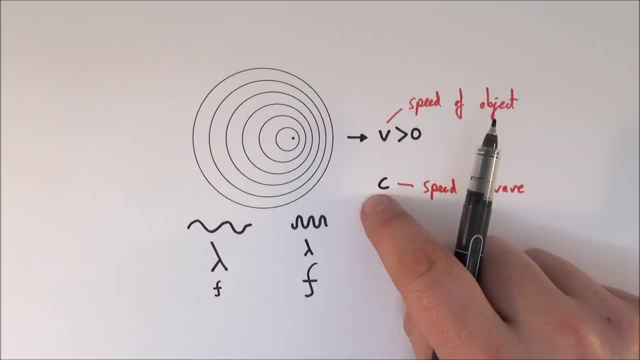 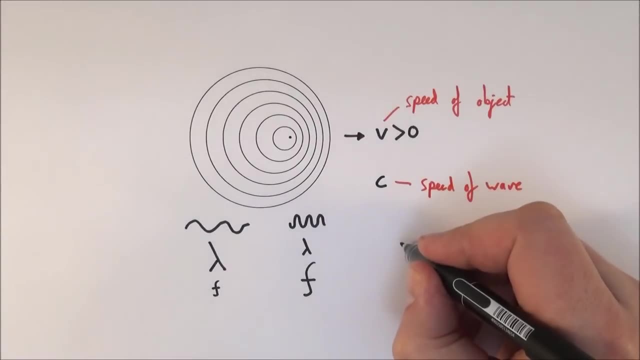 Now, normally we use little c to represent the speed of light, but in actual fact we can use c to be the speed of any wave, And you might see that as the course kind of develops. So what do we know? Well, basically, if we look at the ratio between the speed of the moving object and the speed of the wave, 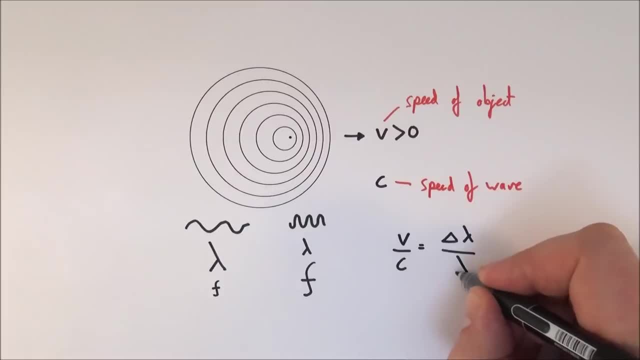 it tells us about the change in wavelength over the original wavelength of that emitted wave. We can also see the same thing: that v of c is also equal to the change in frequency over the original frequency of that wave. Now, these are both approximates and these only work for when we have things which are non-relativistic. 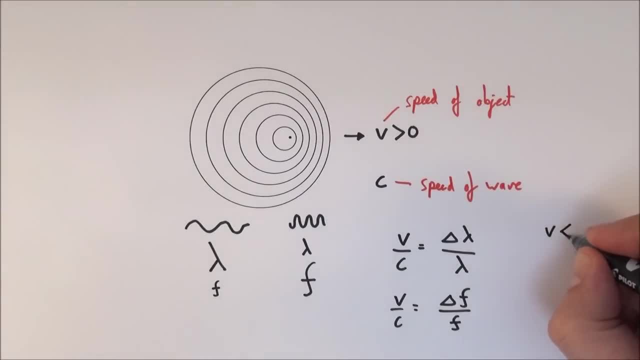 So what we're talking about is the speed of the object is going to be a lot smaller than the speed of light, And that means we can just look at non-relativistic effects. There's another formula for when we look at special relativity. 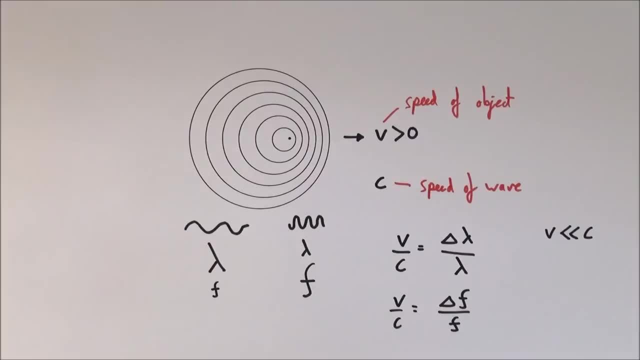 And how that affects things, but that's just way beyond what we need to know at the moment. The other thing that you might be interested in knowing is that we can also give this ratio of v over c the letter z, where z is equal to v over c. 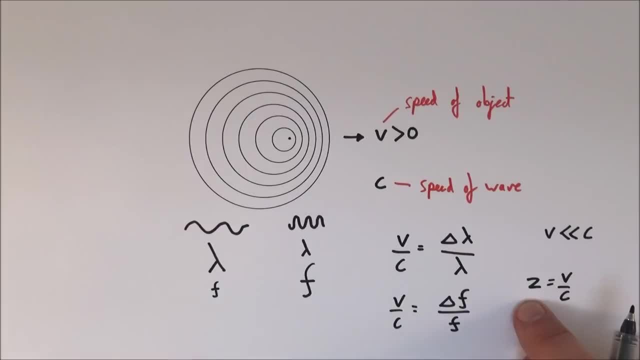 And this is really useful when we're looking at astronomy And if we're looking at the redshift of stars. so what we're talking about is light emitted from a star. If the star's moving very quickly, then we get. if the stars or galaxies are moving towards us, we get a blue shift in the light in it. 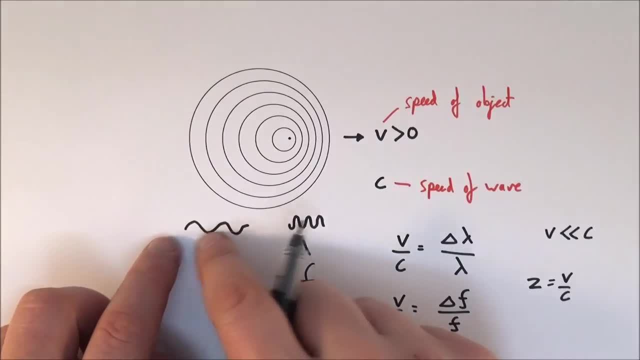 We get a shorter wavelength. If it's moving away from us, the light is stretched out towards the red end of the spectrum And then we get a redshift in that light, or especially the Doppler shift of spectral lines. We can then give us a value of z. 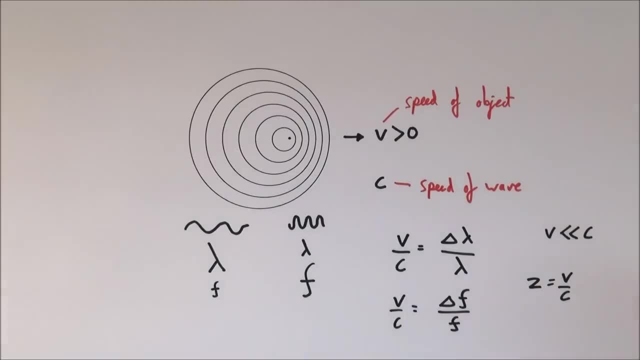 Well, that basically tells us how fast something is moving away. So why is the Doppler effect important? Well, there are three main areas that it's used for. We have already talked about it just then. But what we're looking at is the redshift of galaxies moving throughout the universe.